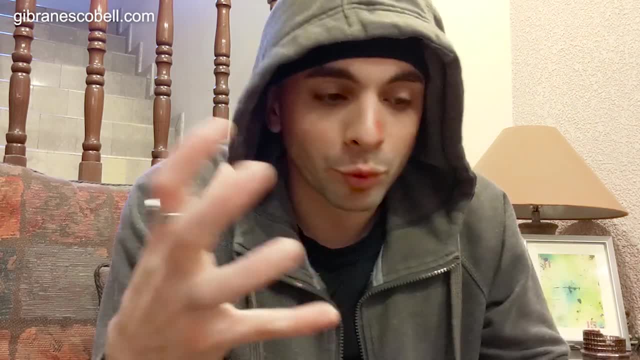 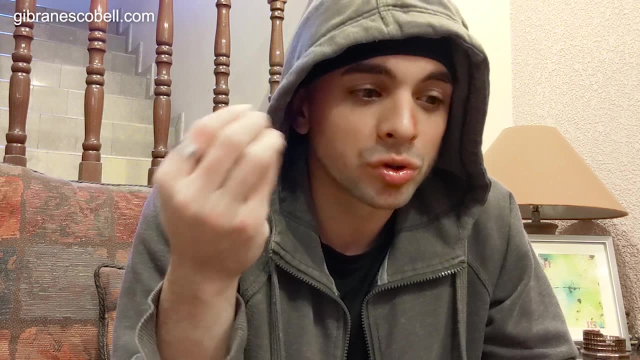 to be in your brain. You know how we have this little voice in our brains. Everyone has this little voice right there. When you're just like blank- you know you're not thinking of anything- this voice will come out and try to tell you things, right? Well, whatever comes out in this, 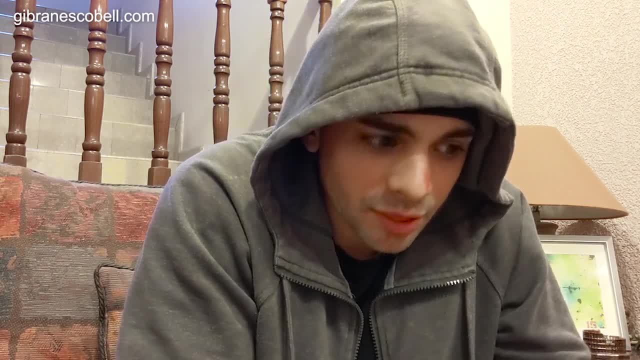 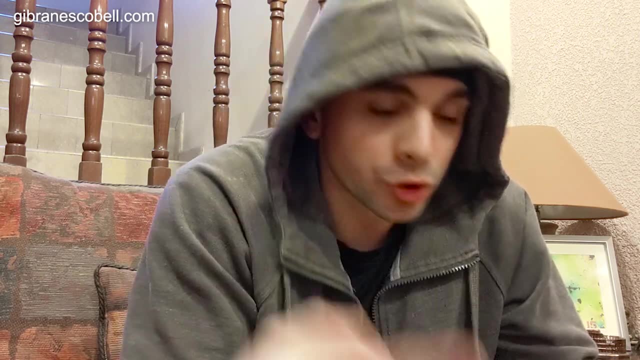 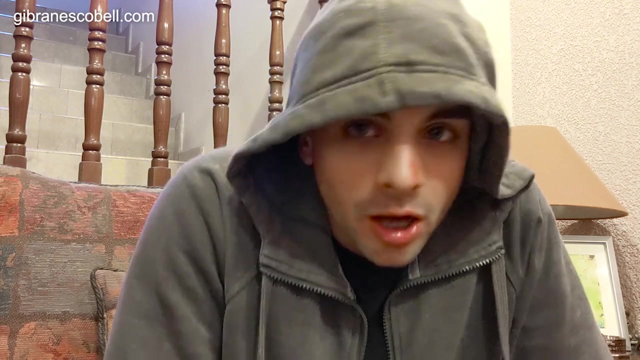 voice that you hear, that everyone has inside their heads. that voice or whatever those thoughts are a matter of repetition. You've consistently repeated something over and over and now it's a habit. So people that have a lot of negative thoughts and negative emotions it's because 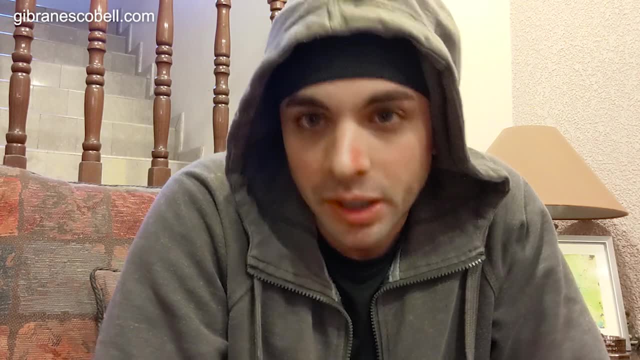 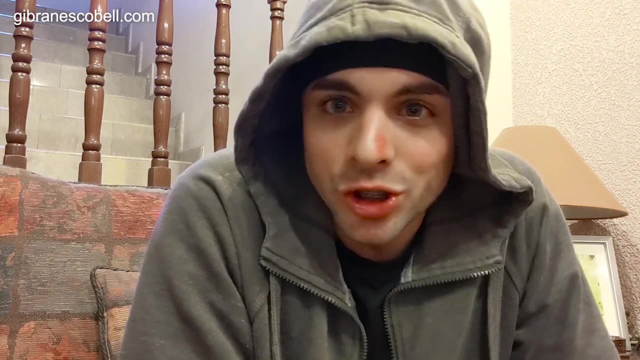 they've worked consistently and repeating themselves something negative over and over and over and over again. So because your brain is trying to optimize and not spend more energy, it's going to bring that thought out, That negative thought. if you tell yourself: I don't know. 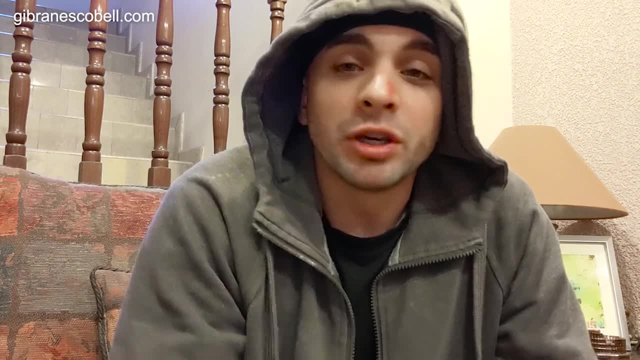 oh, I don't like my skin color, for example. right, And you keep saying to yourself: I don't like my skin color, I don't like my skin color, I don't like my skin color. Well, when you stop thinking, 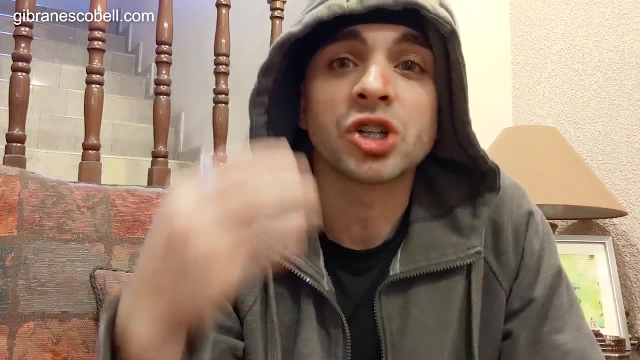 of that. it's going to come out. This thought is going to come out and it's going to start telling you: I don't like my skin color. So now, because you're thinking that way, you're going to start feeling that way and you're going to create a negative thought And that's going to bring 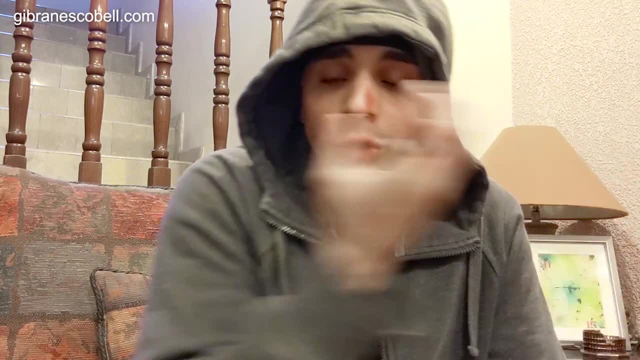 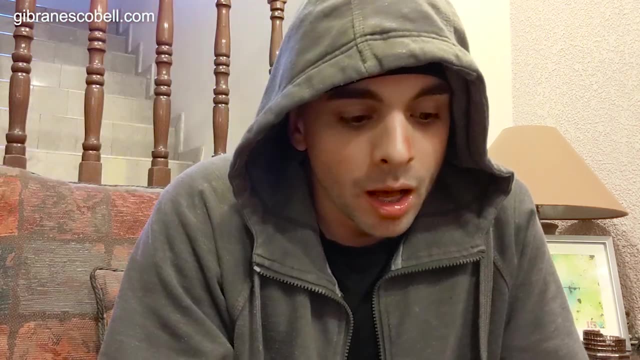 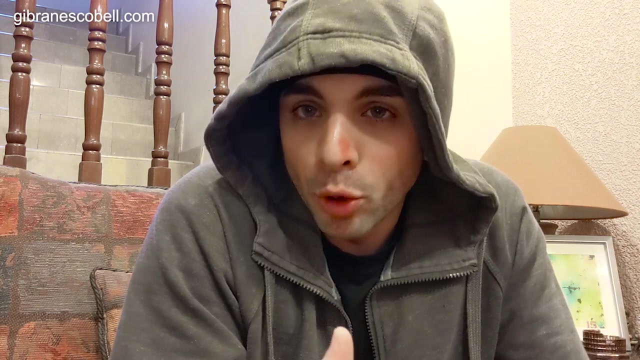 these emotions? right. So the thoughts will create the emotions, but it all starts with how you think and the repetition. that is called auto-suggestion, right? Auto-suggestion is when you repeat something over and over, it becomes automatic. It's auto-hypnosis, basically. And 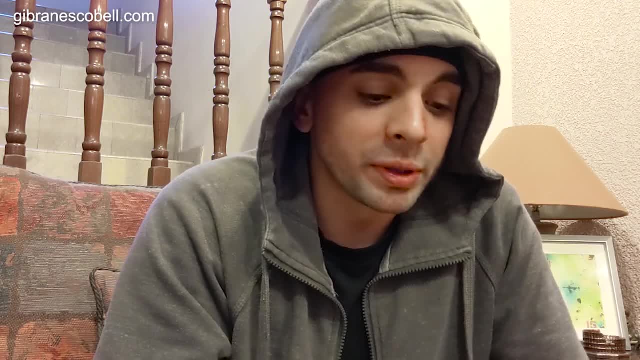 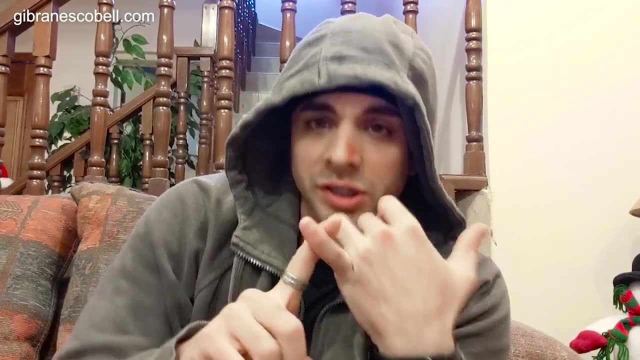 that's how hypnosis works. So you repeat something over and over and over and it will become consistent over your head because you're creating a connection, a habit. So the question is: positive affirmation, Positive self-talk: Do they work? Yes, they do, Because you're repeating something over and over. 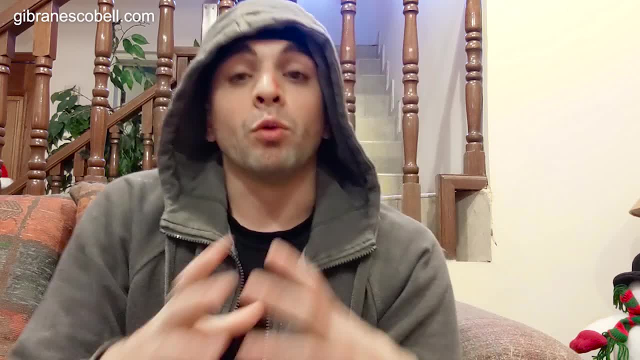 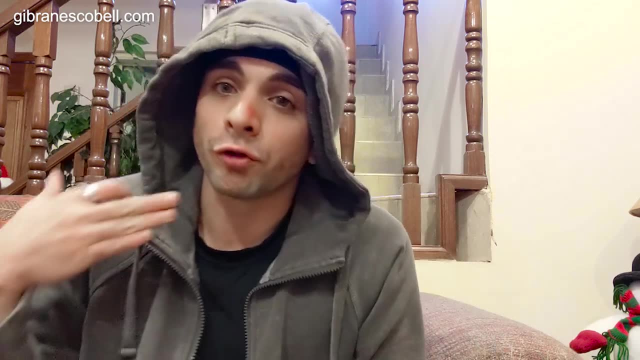 and you're creating a habit in your brain. So that way, maybe, when you're feeling down, when you're not feeling like you're in a happy place, those positive thoughts which you've created through habits, they will come out automatically and help you and they will boost the way you feel. 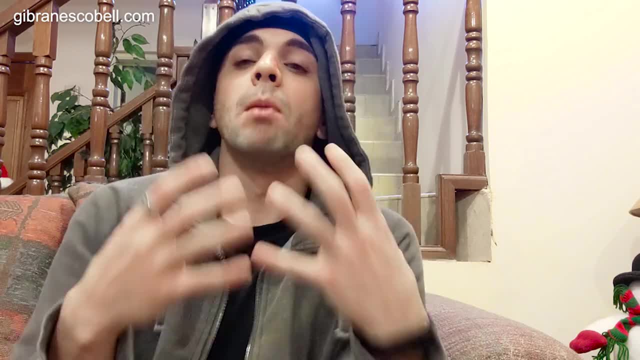 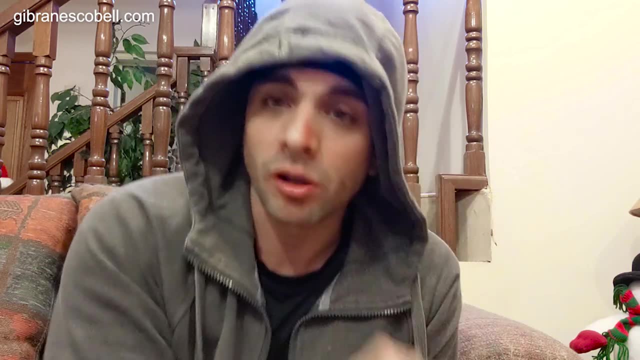 So what you have to do from now on is you have to monitor your thoughts and change the negative thoughts to positive thoughts, Because by changing that and then repeating yourself positive things, which is the positive affirmations right And the positive self-talk, by repeating that over and 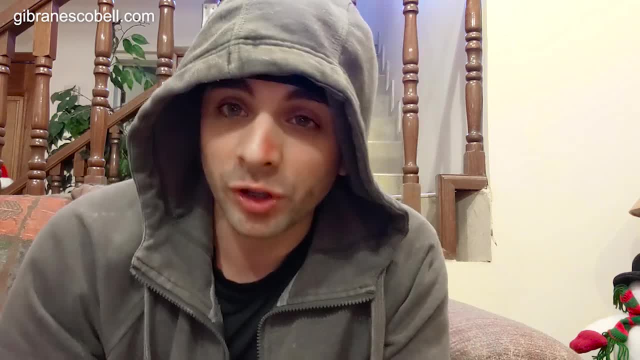 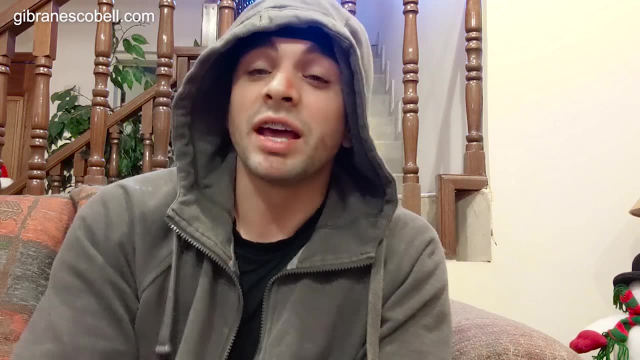 over. you're creating a connection And, once again, when you're feeling down, they will lift you up, They will lift your mood. So, on the other hand, if you're telling yourself negative things, negative self-talk, thinking negative things about your environment or yourself or whatever, 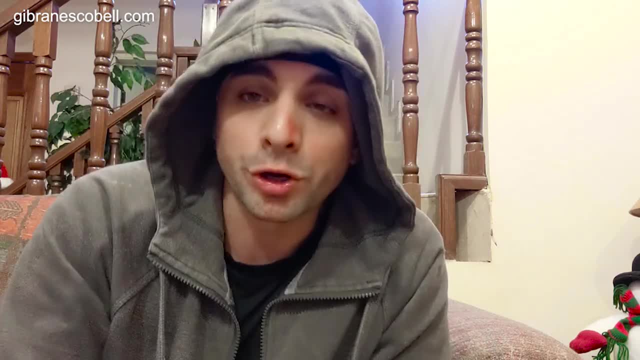 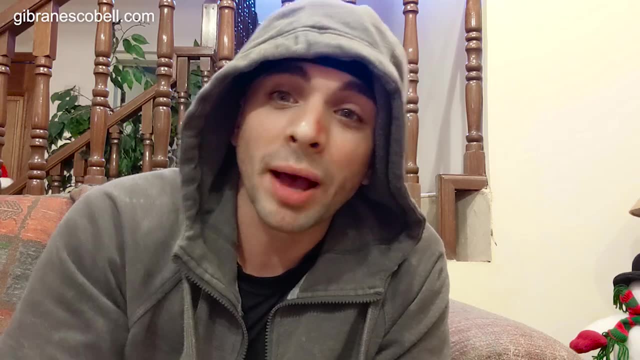 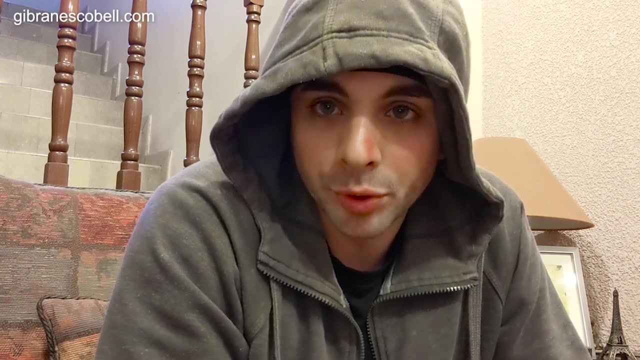 or about other people. repeating that over and over will bring that out. So if you're already feeling down, they will pull you down even more because they will come out automatically. I want you to think of this this way: Imagine you're teaching a parrot to talk- A bird right. A parrot repeats what you tell. 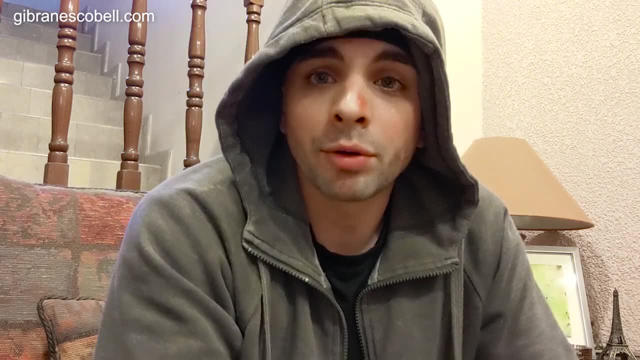 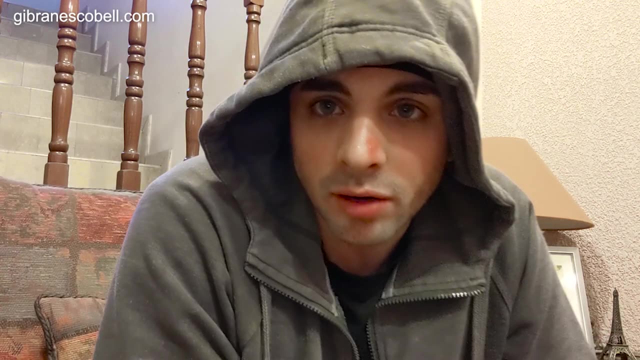 So if you're teaching the parrot positive words, the parrot is going to repeat back to you those positive words, because that's the language the parrot knows. If you teach the parrot negative words and negative things, the parrot is going to repeat back to you negative things. That's the same way. 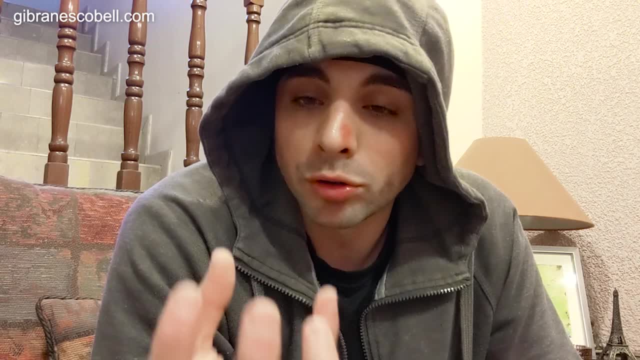 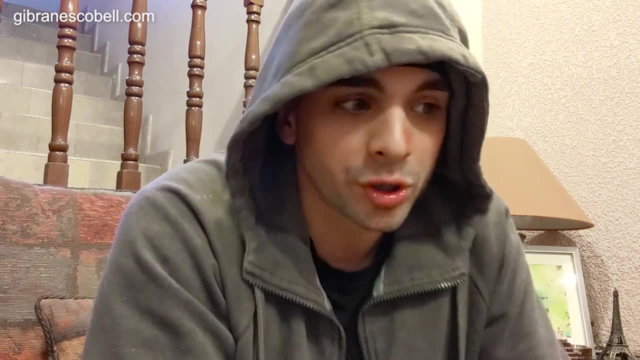 your brain works Like a parrot. you teach your parrot good, positive words. it's going to repeat back to you positive words. You teach your parrot negative words, it's going to repeat back to you negative words. And you obviously want to be surrounded by a parrot that is going to tell. 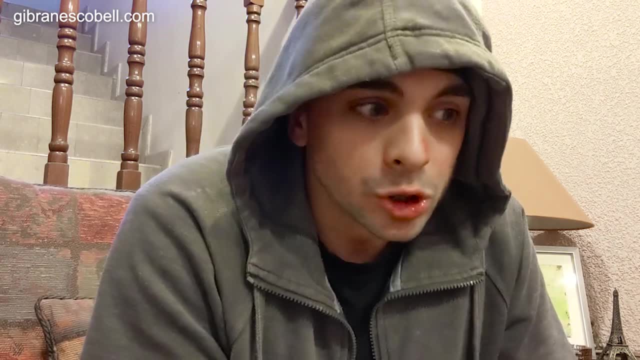 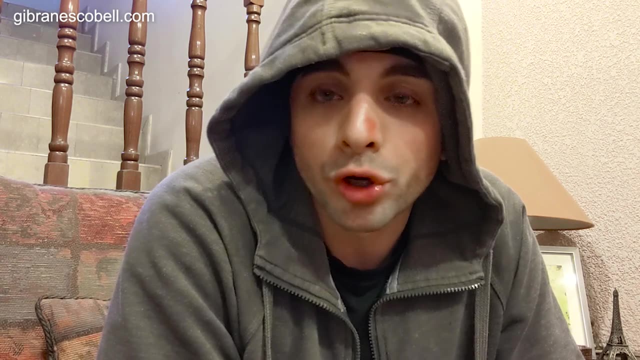 you positive things. No one wants to be around a negative person, right? So that's how your brain works. So positive affirmations: do they work? Yes, they do. Positive self-talk: it also works. Telling yourself negative things. if you're having negative emotions, you are. 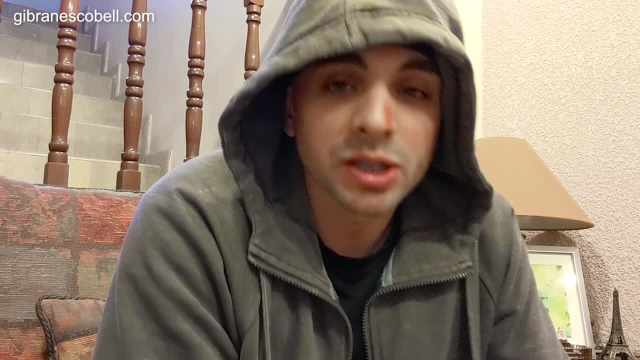 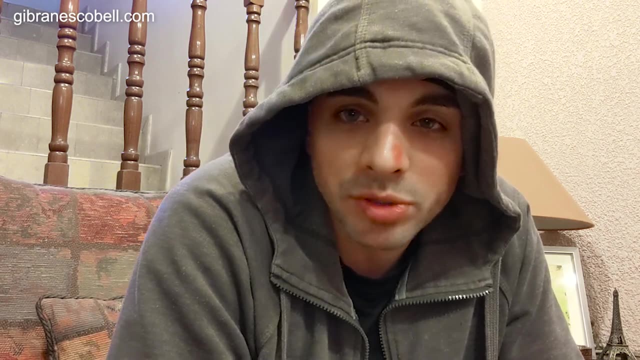 struggling with those negative emotions and those negative thoughts because you're repeating yourself that over and over. You need to distract yourself and start thinking positive- basically That's what it all comes to- And start building those new habits right. Personalities can be modified. 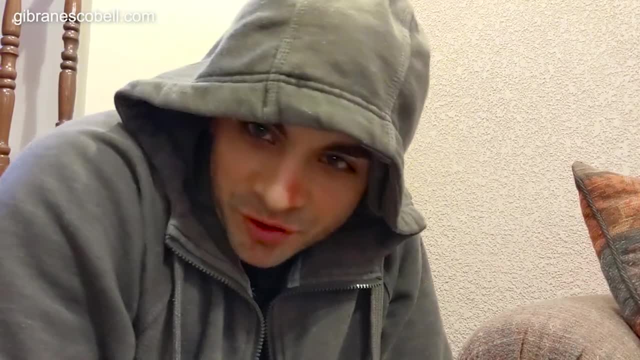 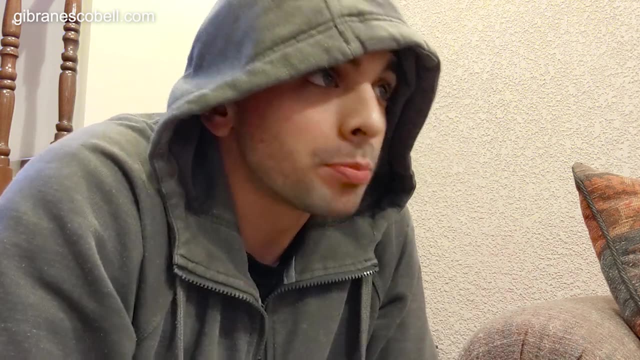 by changing old habits. If you enjoyed the video, make sure you like, comment and subscribe And hit the little notification bell next to the subscribe button, because every week I put a couple of videos out And if you want to get notified when I put those videos out, you need to hit that.